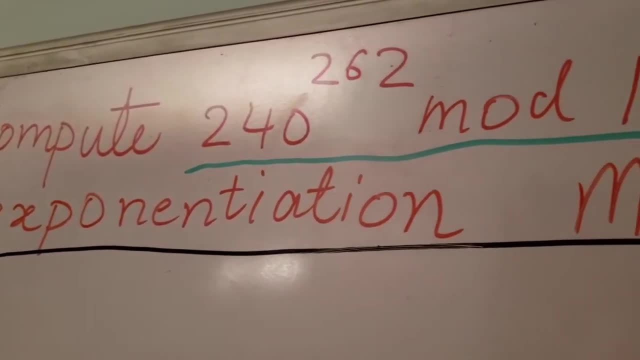 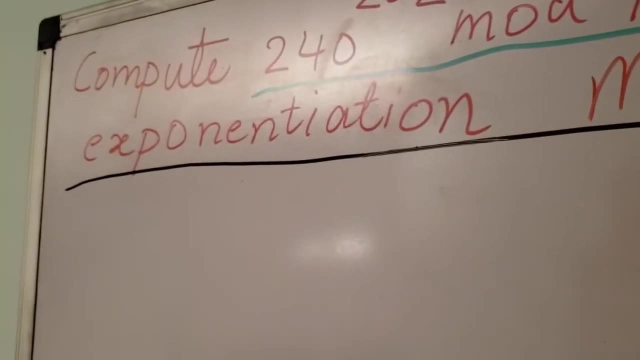 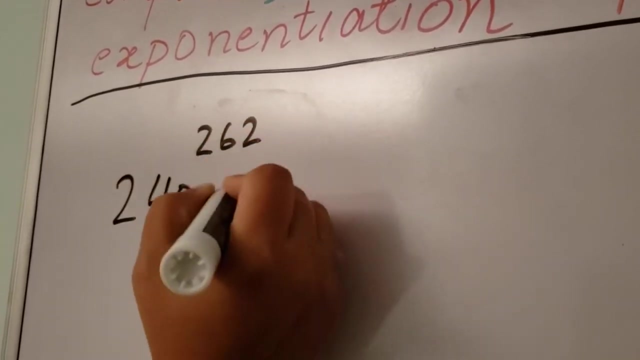 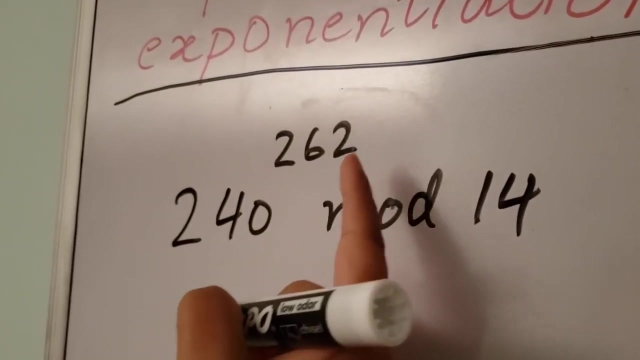 So let's compute 240 to the power of 262 mod 14, using past modular exponentiation method. So let's write down our question: 240 to the power of 262 mod 14.. 240 is our base and 262 is. 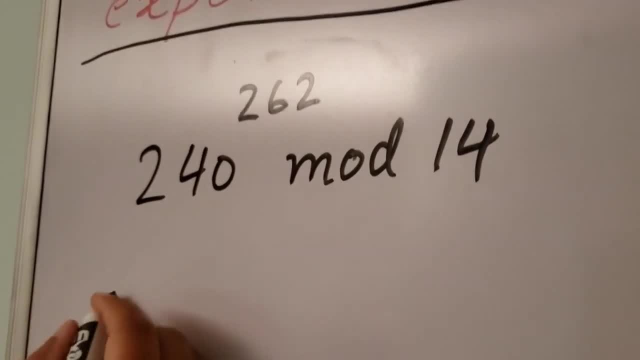 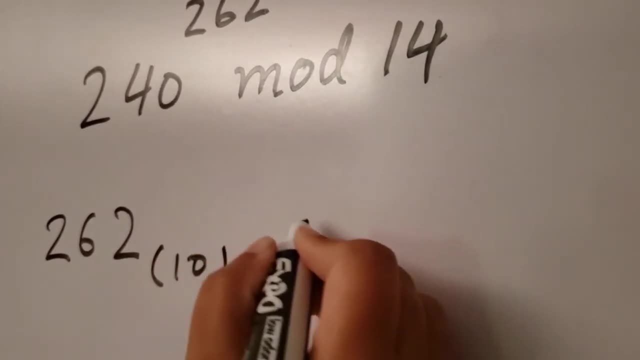 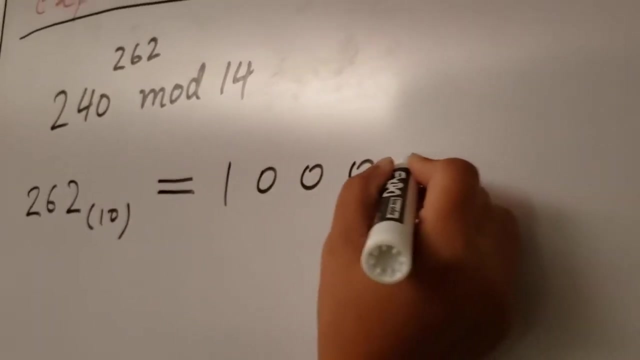 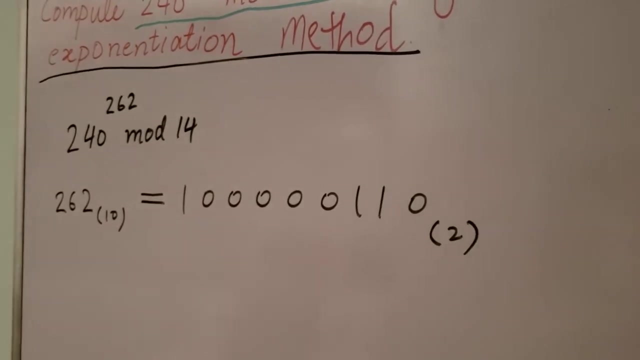 our exponent. The first step is to write down the exponent 262 and find out its binary, which is 1 0 0 0 0 0 1 1 0.. You can easily find out the binary of 262 by decimal to binary conversion. 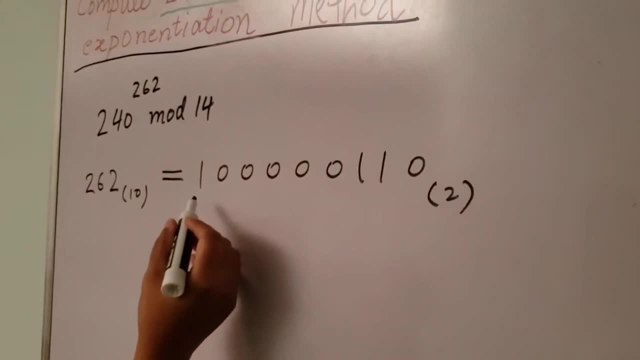 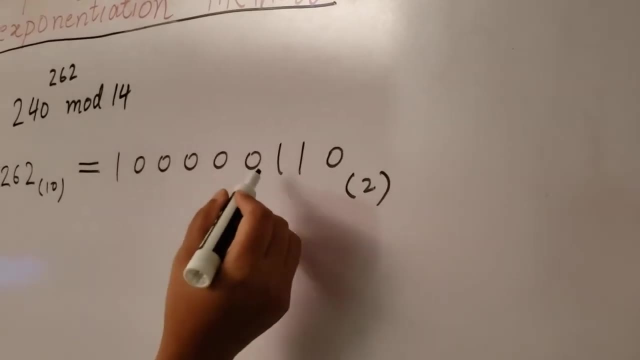 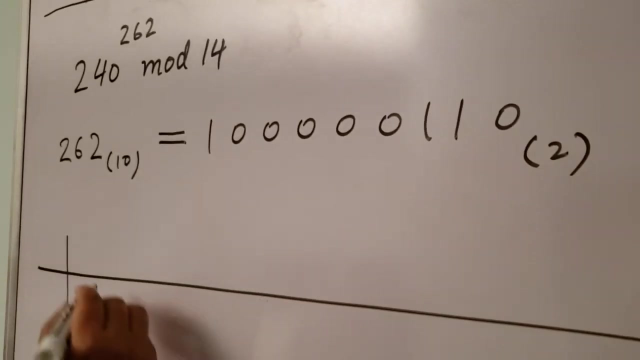 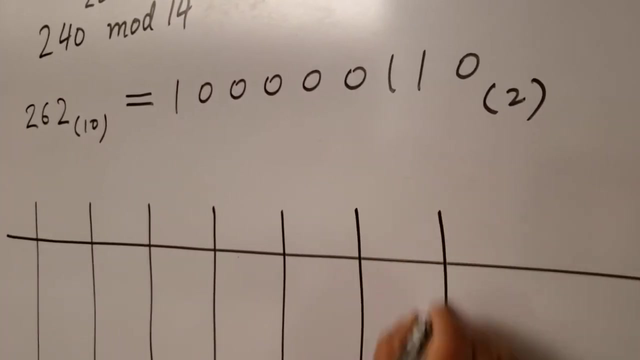 Our next step is: let's count how many binary digits are in this binary number: 1, 2, 3, 4, 5, 6, 7, 8, 9.. Let's draw a table of nine columns: 1, 2, 3, 4, 5, 6, 7, 8, 9.. 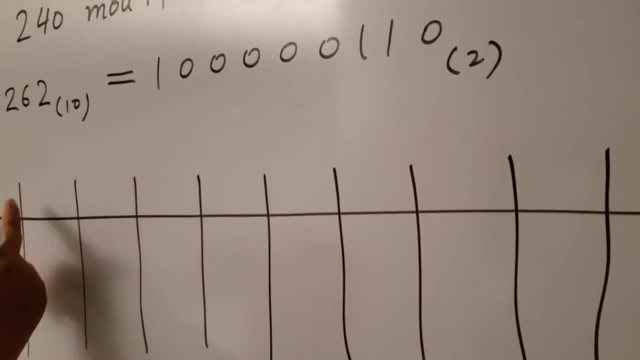 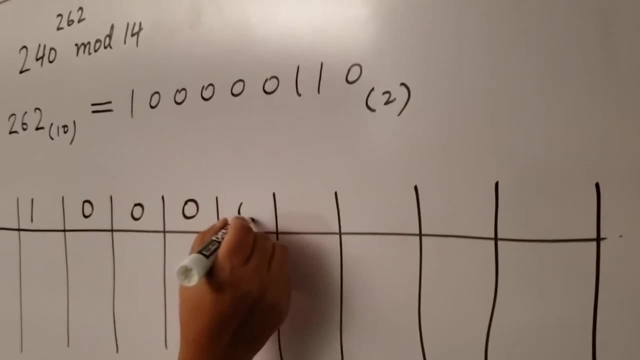 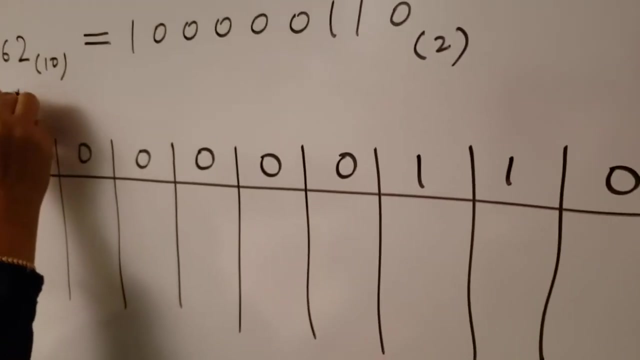 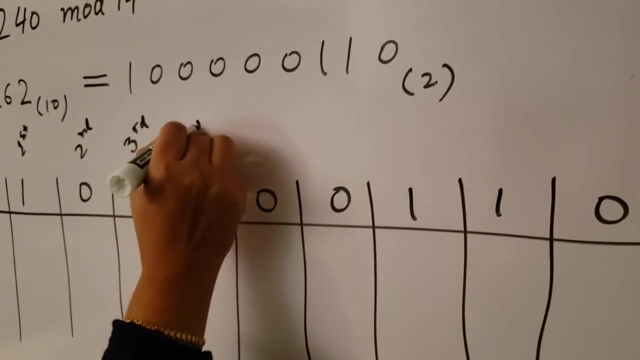 And write down each binary digit on top of this column. Name this column as 1st, 2nd, 3rd, 4th, 5th, 6th, 7th, 8th, 9th, 10th. 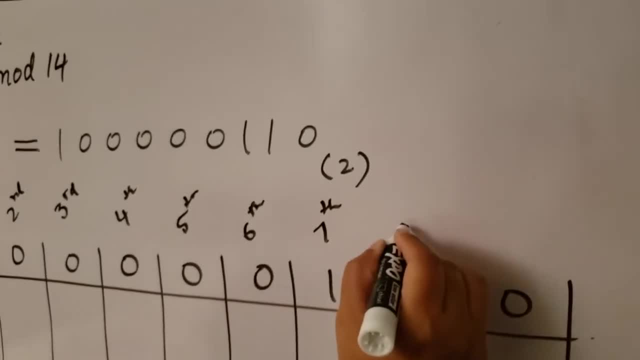 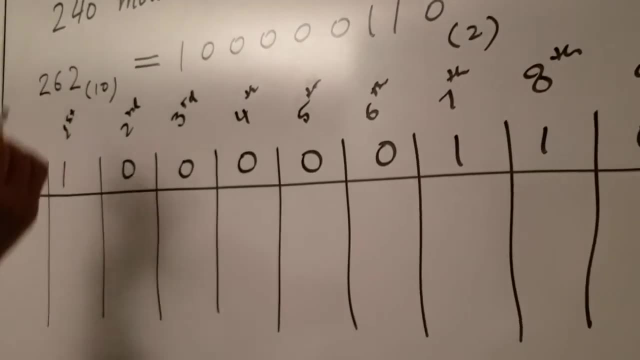 Let's write down our question: How many binary digits are in this binary number One, two, three, four, five, six, seven, eight, nine, ten, seventh, eighth, ninth. okay, so write down the base, which is 240 in our first column. 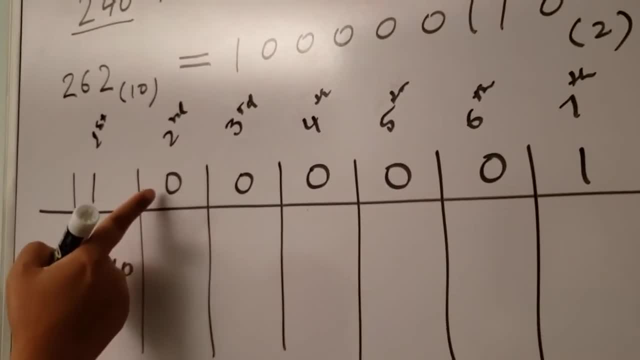 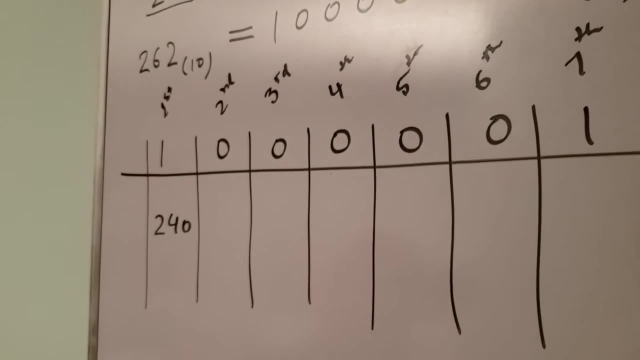 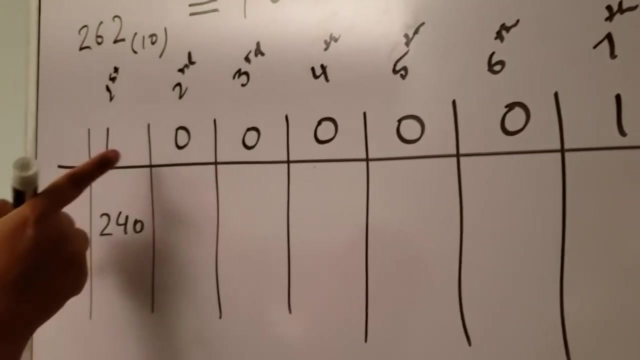 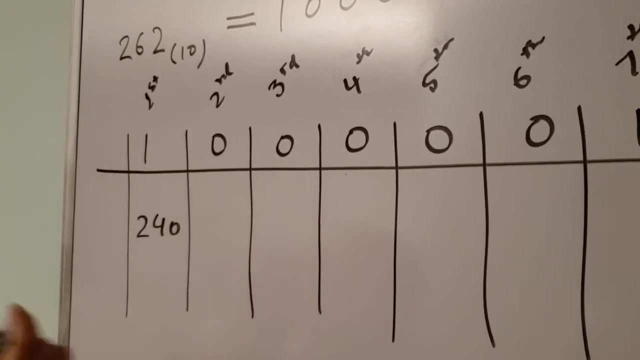 and now look at the binary digit of second column, which is zero. if the binary digit is zero, we have to do only one step, and if the binary digit is one like this, we have to do two steps. we'll see how. let's start working on the second column value, where the top binary digit is zero. 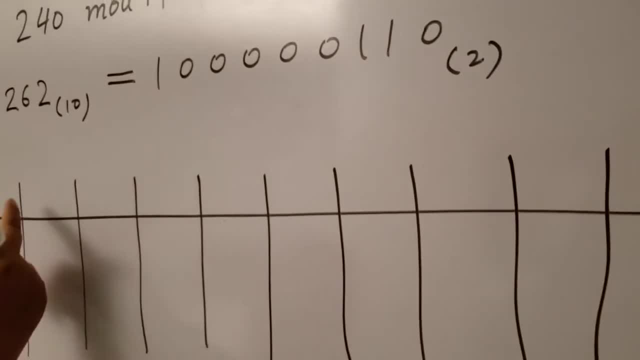 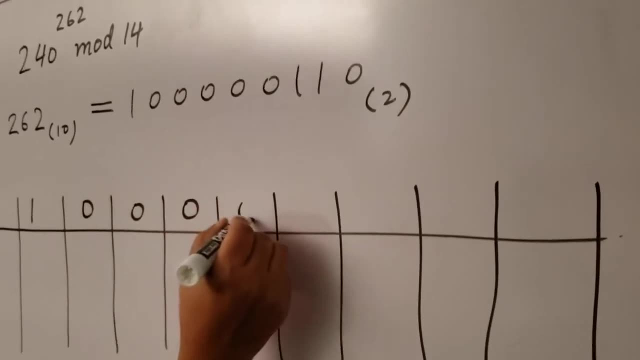 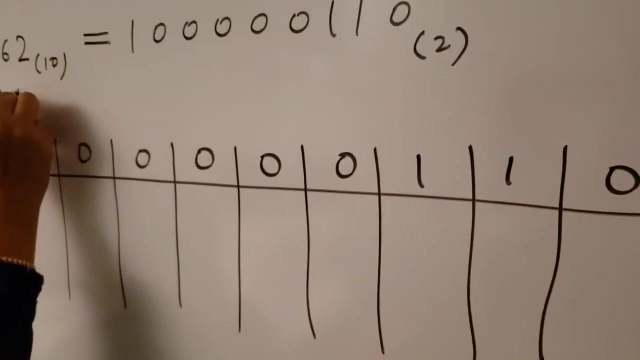 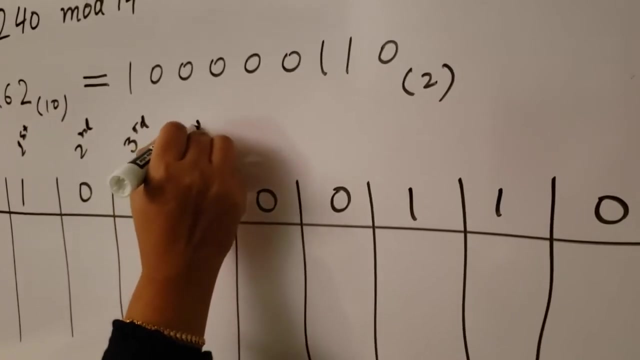 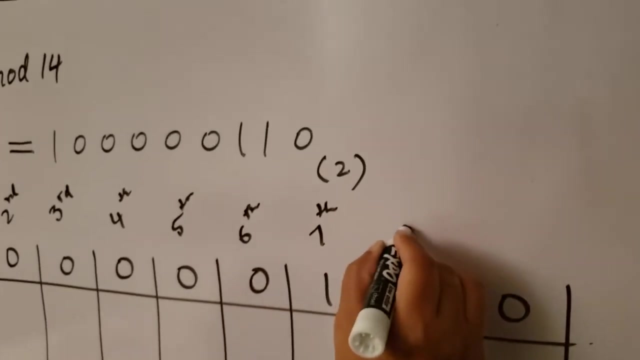 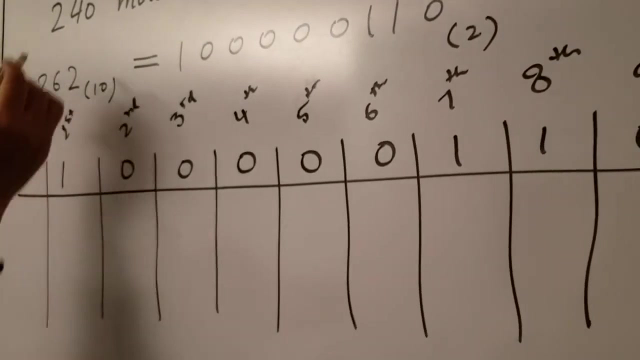 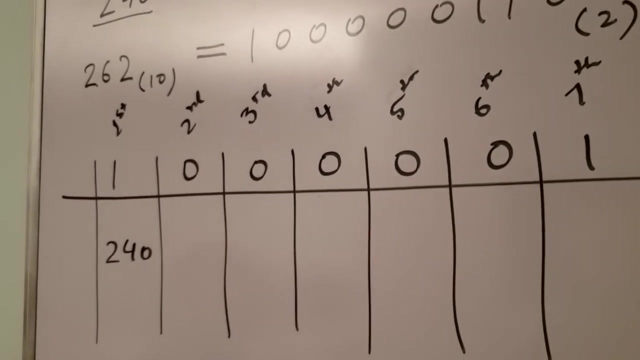 And write down each binary digit on top of this column And name this column as 1st, 2nd, 3rd, 4th, 5th, 6th. so write down the base, which is 240, in our first column, and now look at the binary digit of second. 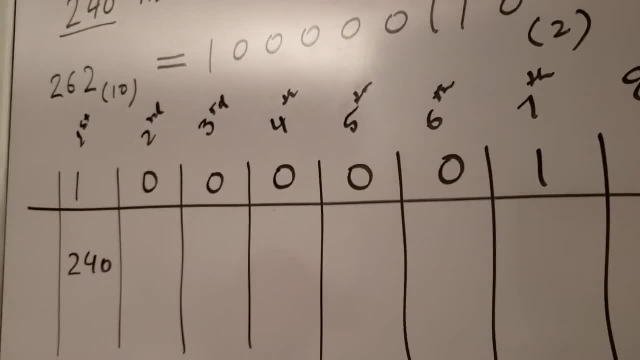 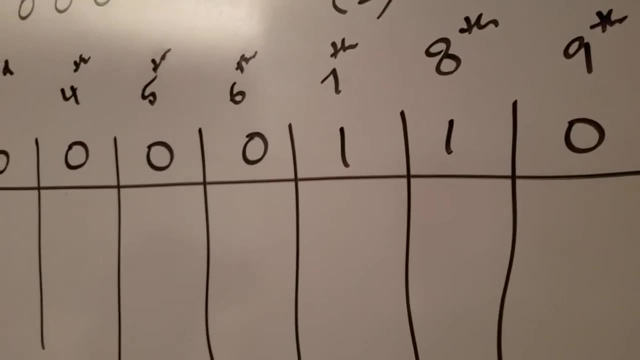 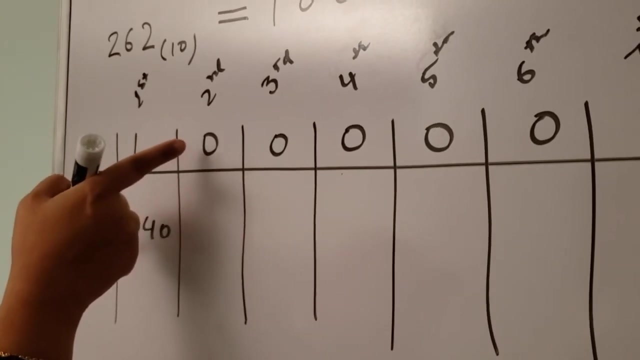 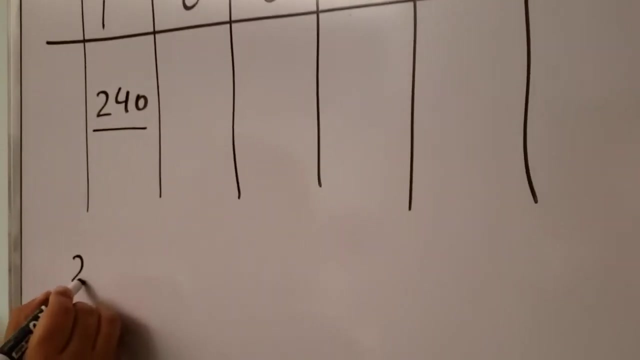 column which is 0. if the binary digit is 0, we have to do only one step, and if the binary digit is 1, like this, we have to do two steps. we'll see how let's start working on the second column value, where the top binary digit is 0. so take the number from column 1 and square this number and modular. 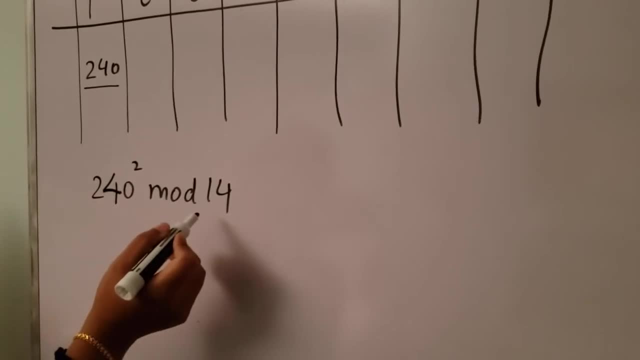 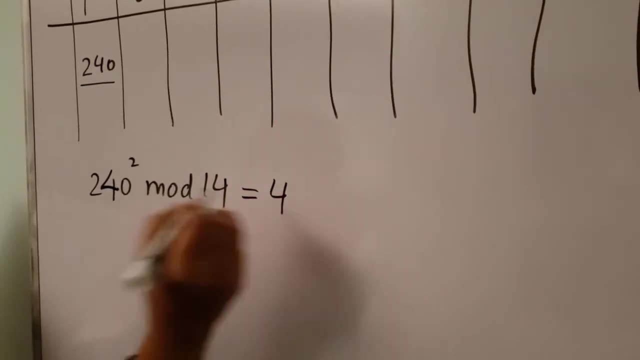 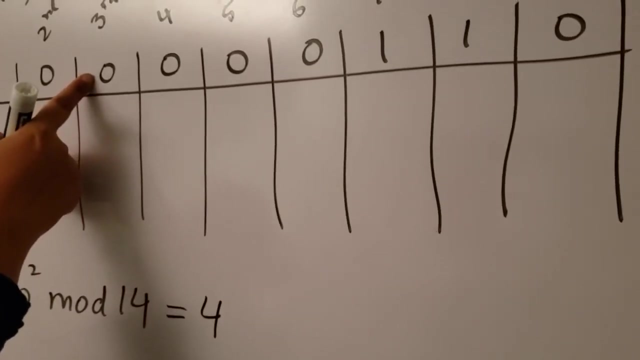 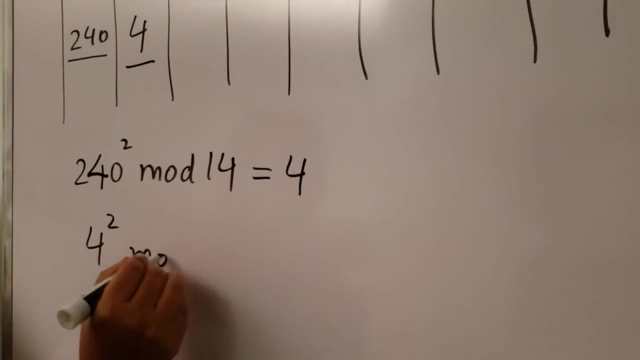 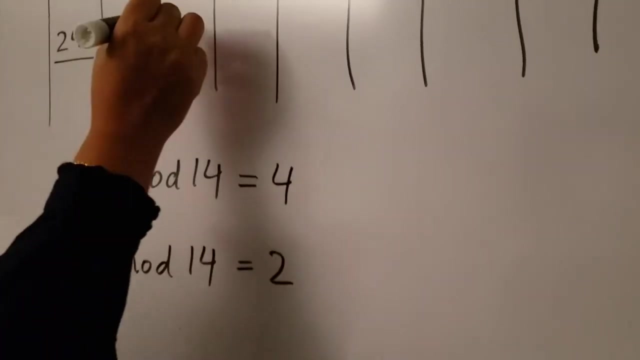 14, the square mod 14, is very easy to calculate it by hand. you won't need a calculator to calculate this. and it is 4. write this 4 in second column. now look at the binary digit of third column, which is again 0. so take 4, square it, and mod 14, which is equal to 2, write 2 in third column. look at the. 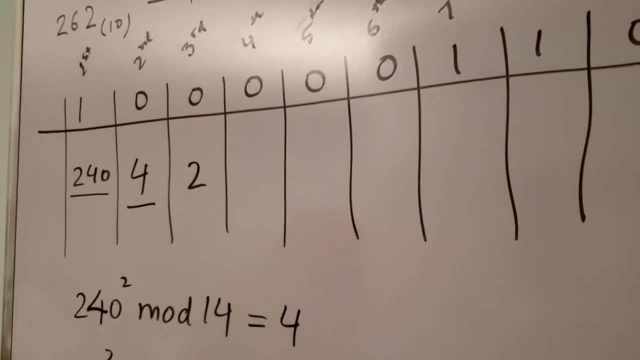 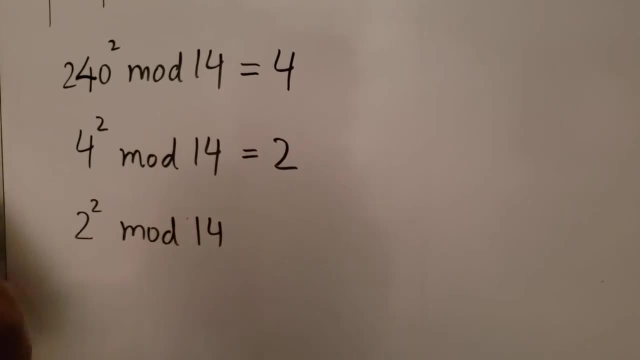 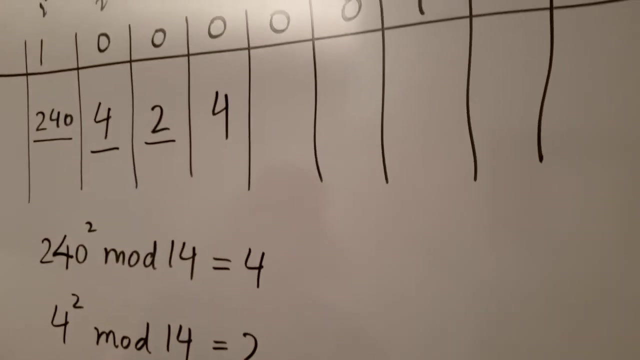 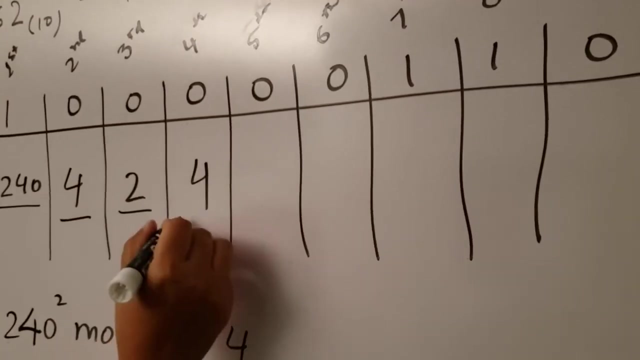 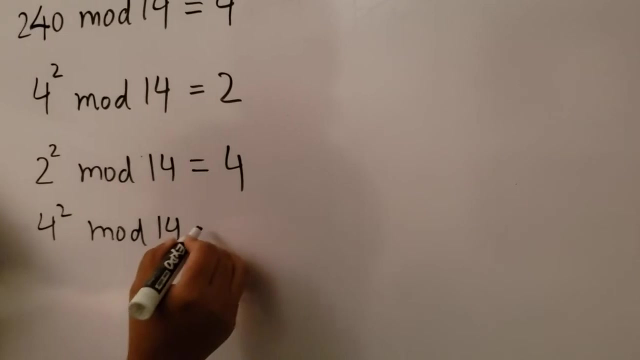 binary digit of fourth column, which is 0. again take 2, square it, and mod 14, which is equal to 4. write 4 in fourth column. let's look at the binary digit of fifth column, which is again 0. so take 4, square it, mod 14, which is equal to 2. 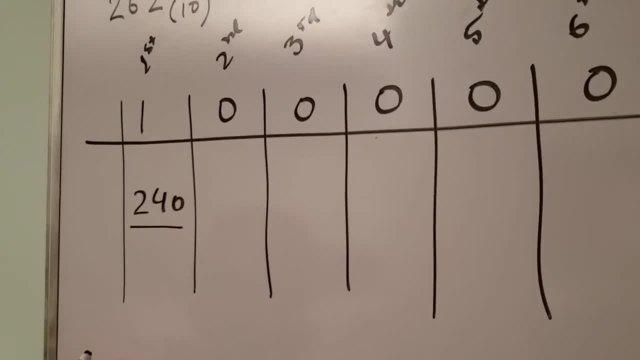 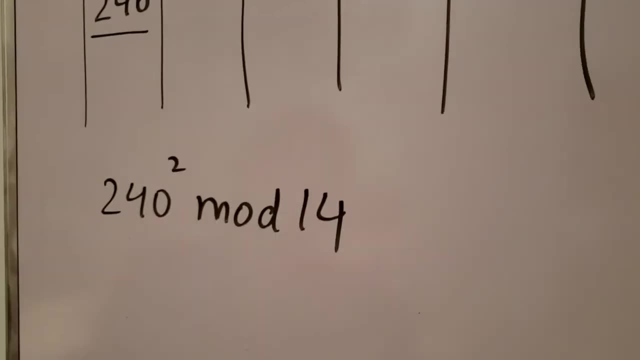 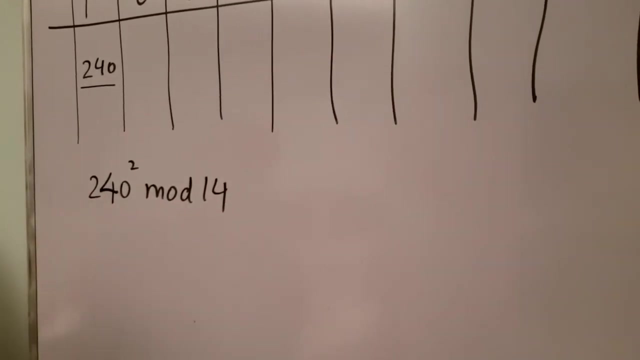 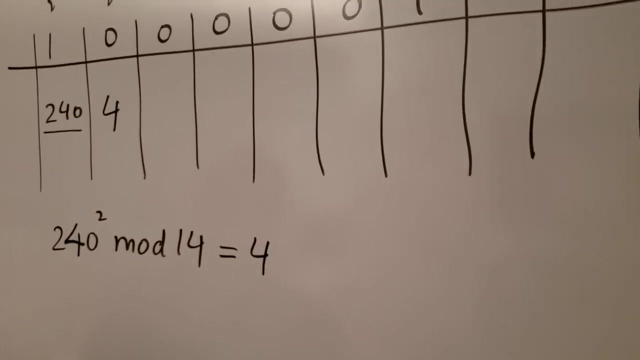 so take the number from column one and square this number and modular 14.. the square mod 14 is very easy to calculate it: by hand. you won't need a calculator to calculate this. and it is four. write this four in second column. now look at the binary digit of third column, which is again zero. so take four. 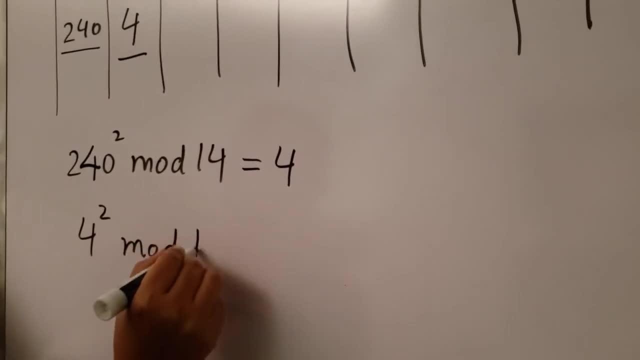 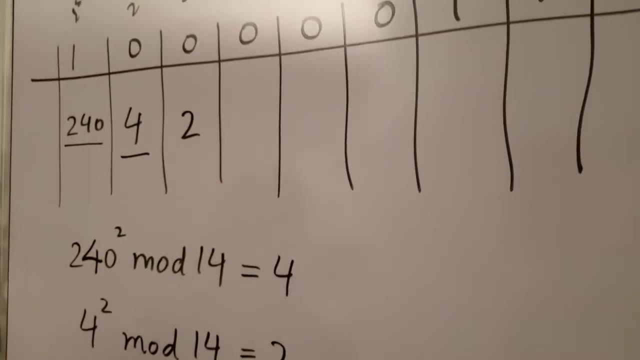 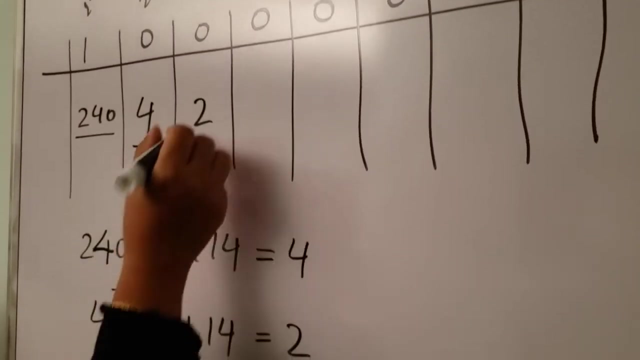 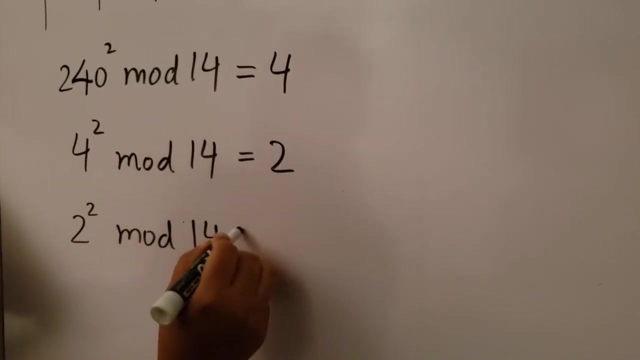 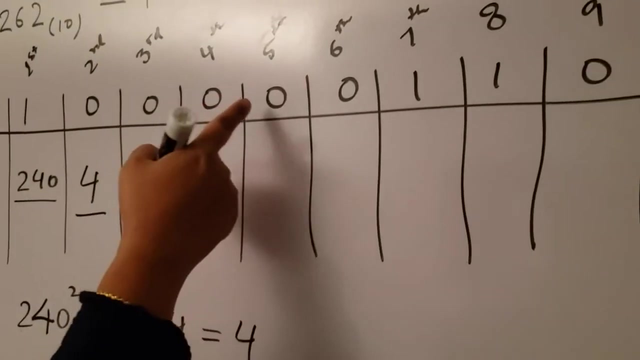 square it and mod 14, which is equal to two. write two in third column. look at the binary digit of fourth column, which is zero. again, take two, square it and mod 14, which is equal to four. write four in fourth column. let's look at the binary digit of fifth column, which is again 0. 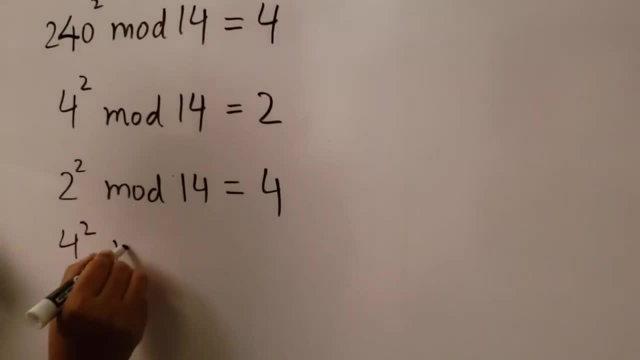 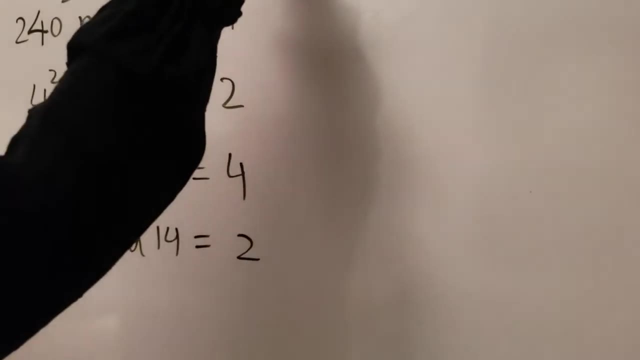 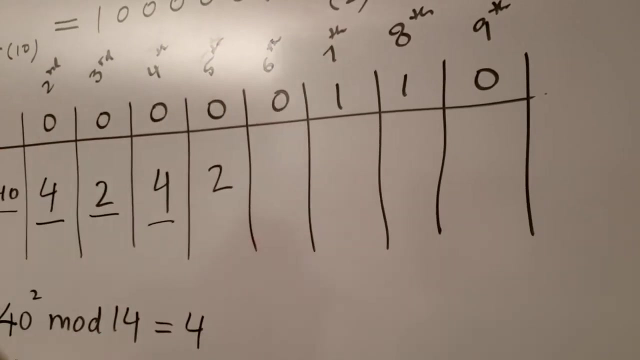 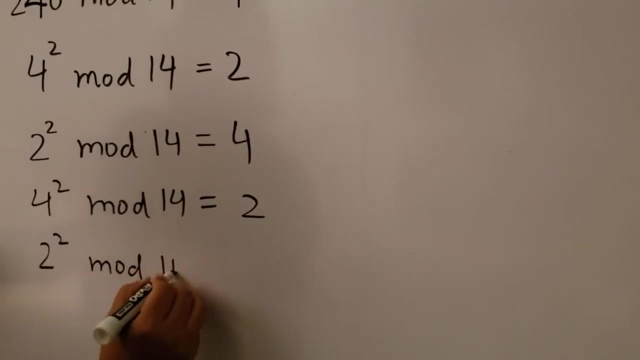 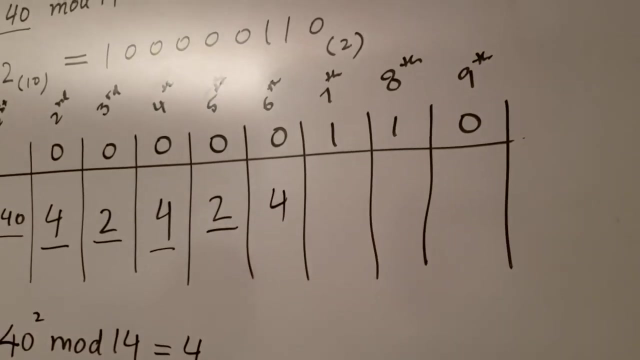 so take four square it mod 14, which is equal to two. write two in fifth column. then let's look at the top binary digit of sixth column, which is again zero. take two square it mod 14, which is four. write down four in the sixth column. now let's look at the top binary digit of seventh column. 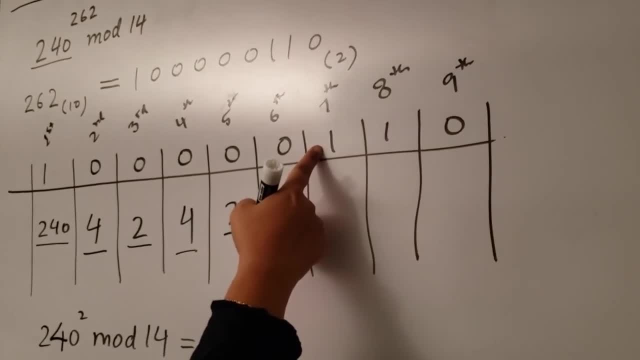 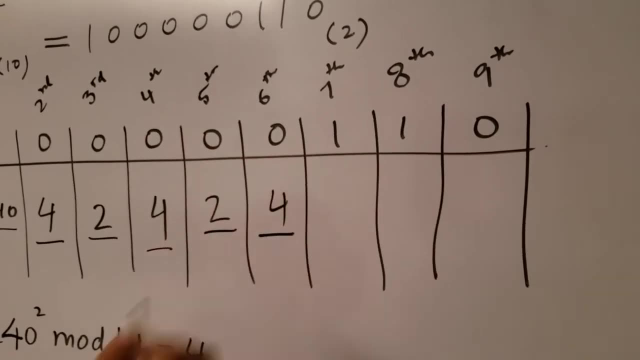 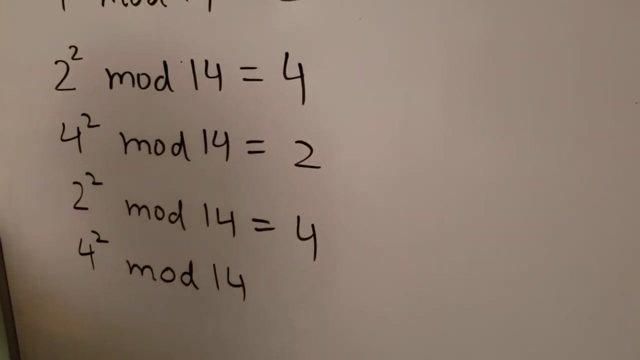 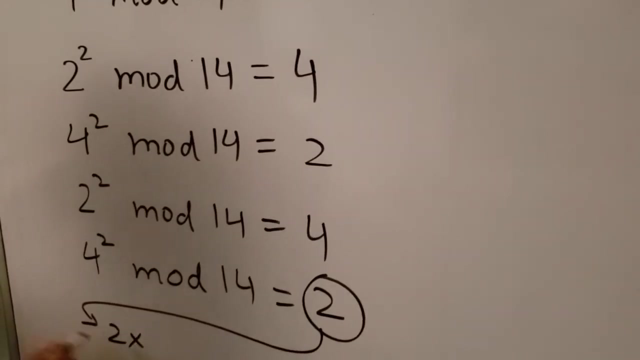 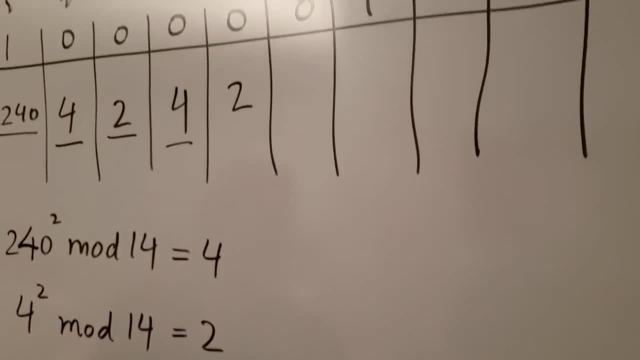 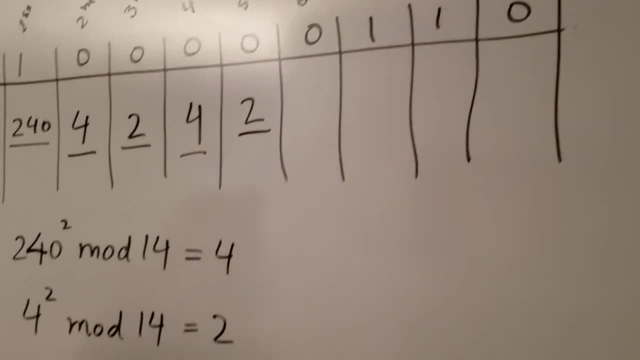 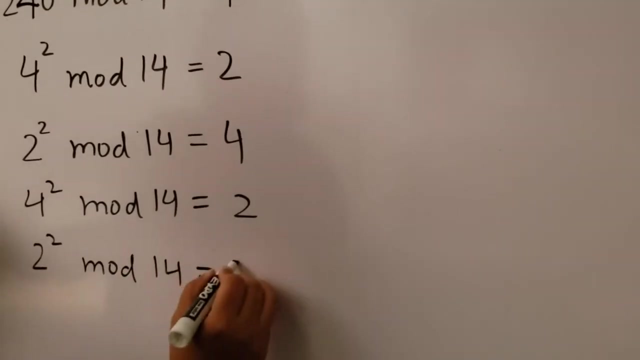 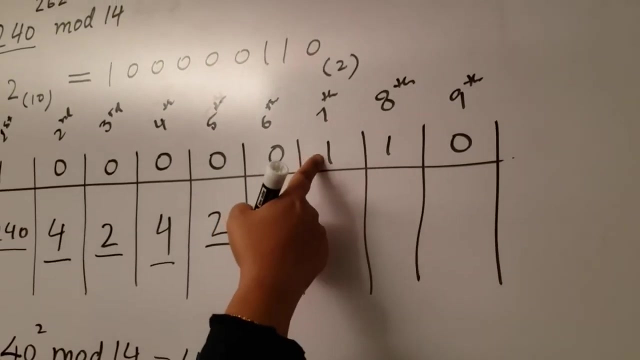 write 2 in fifth column. then let's look at the top binary digit of sixth column, which is again 0. take 2, square it mod 14, which is 4. write down 4 in the sixth column. now let's look at the top binary. 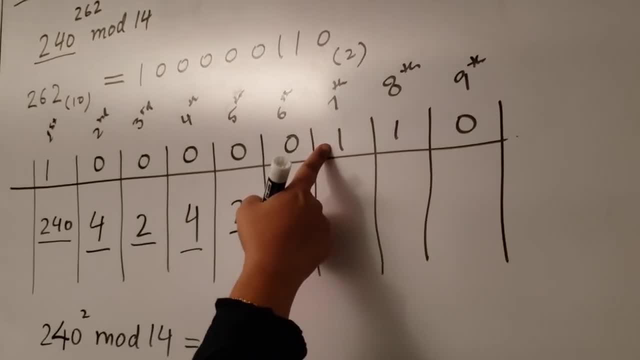 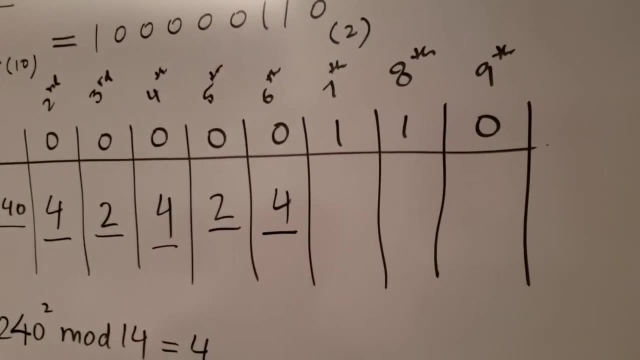 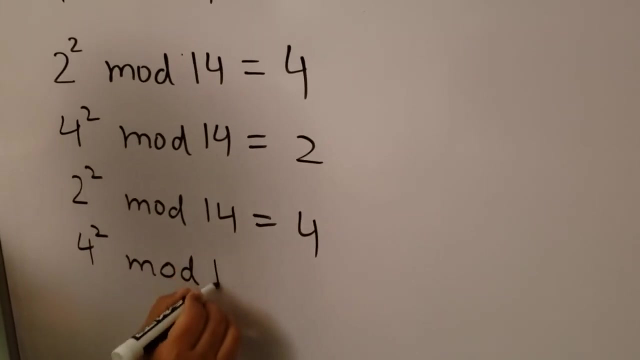 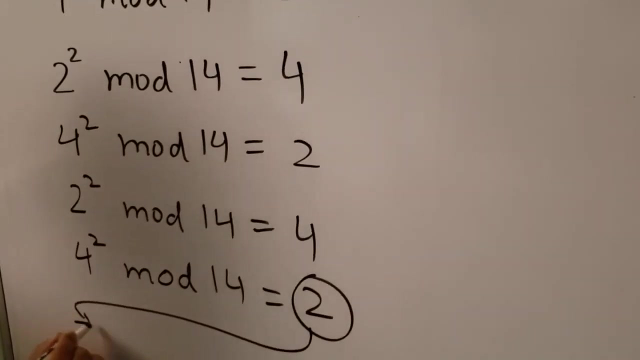 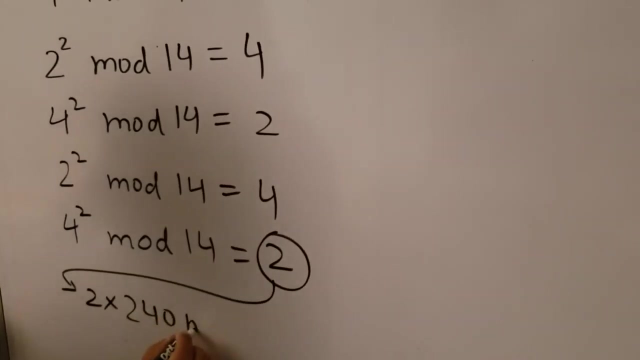 digit of seventh column. now our binary digit is 1. that means now we have to do one step at a time. we have to do two steps. let's see what are the two steps. let's take 4 from the sixth column, again in the same way, square it and mod 14. you will get 2. now multiply this 2 by the base 240 and then mod. 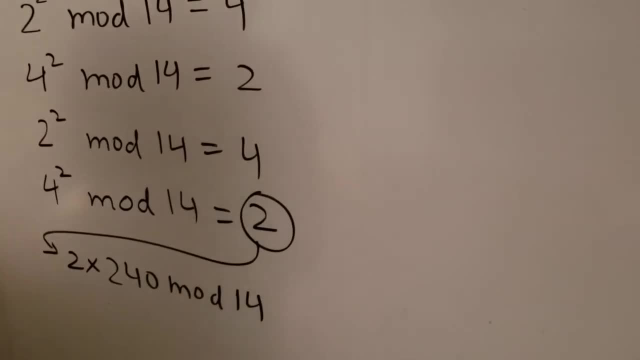 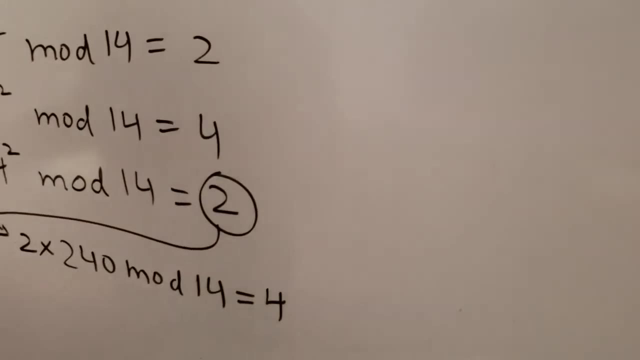 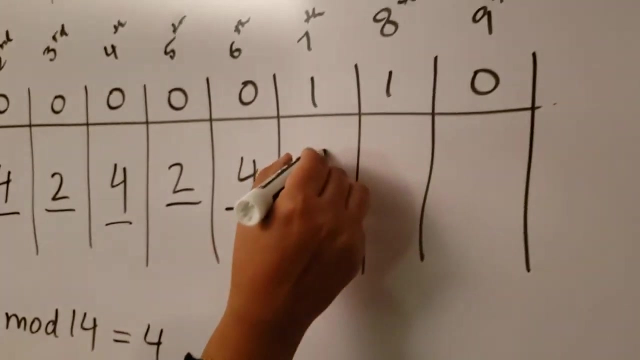 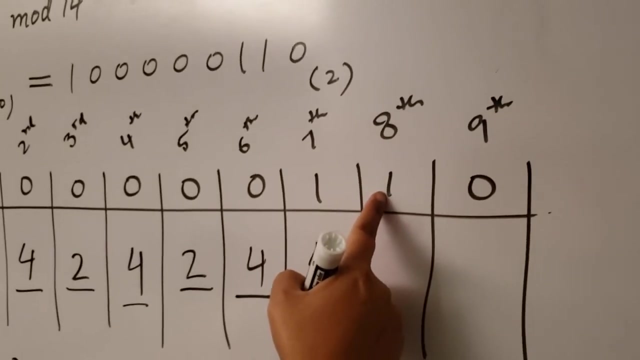 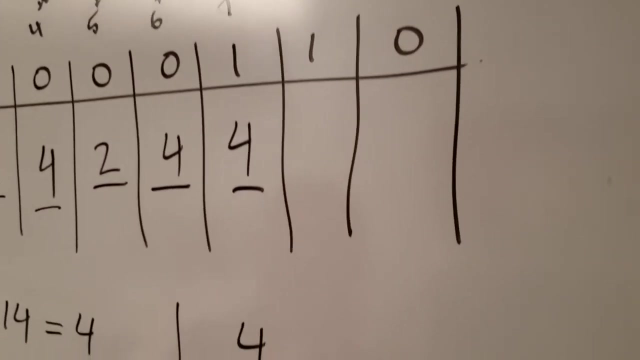 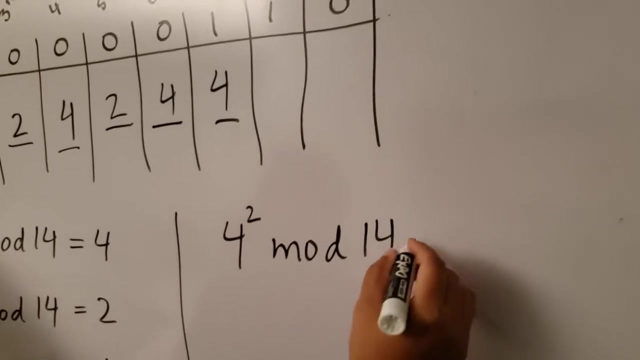 40, you will get the answer 4. so you get the value 4 here. write down 4 in seventh column. now let's look at the binary digit of eighth column, which is again 1. now you have to do the two step in this stage. Take 4 square mod 14, which is equal to 2.. The second step is take this: 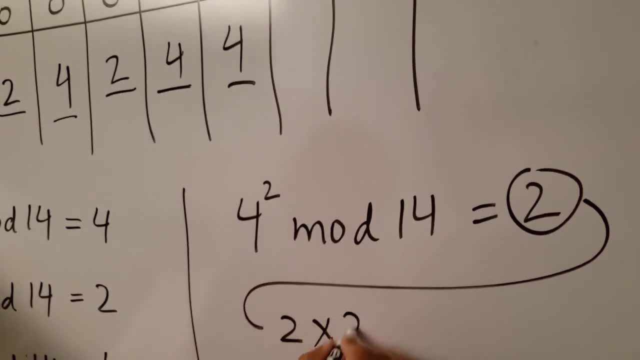 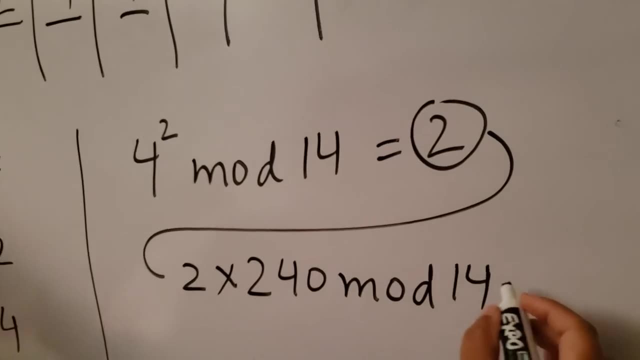 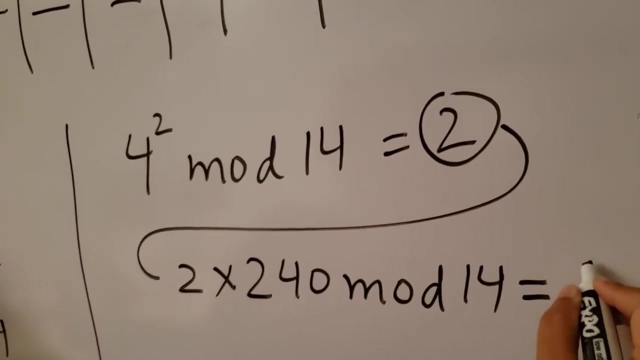 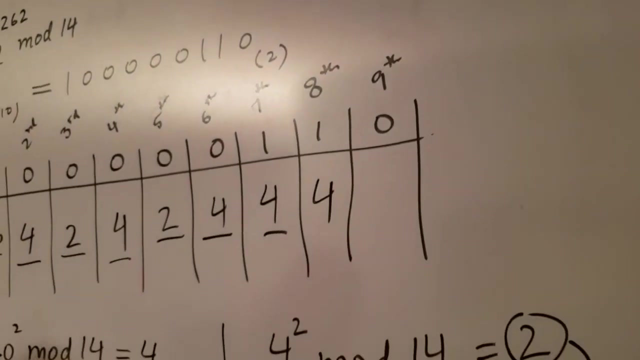 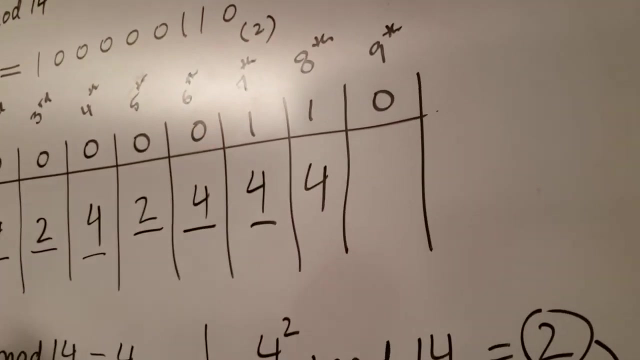 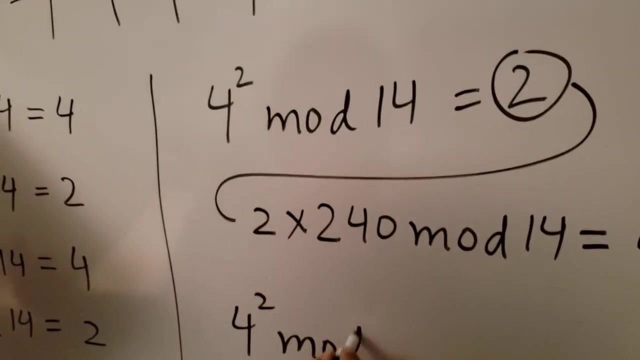 2 multiplied by the base 240 mod 14.. You will get 4.. Write down 4 here. Now let's look at the binary digit of 9th column, which is 0. That means now you have to do one step. Take the value 4, square it mod 14.. You will get. 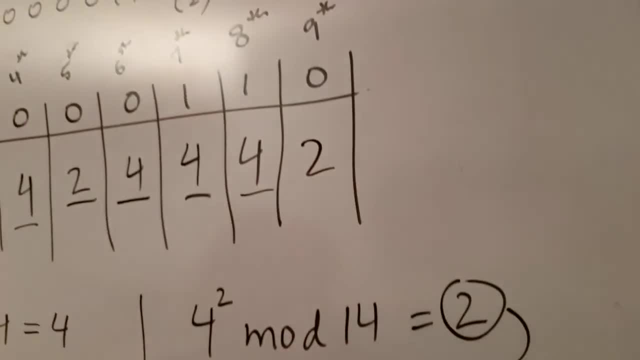 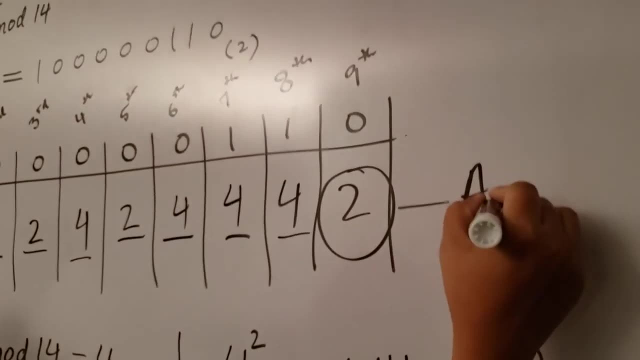 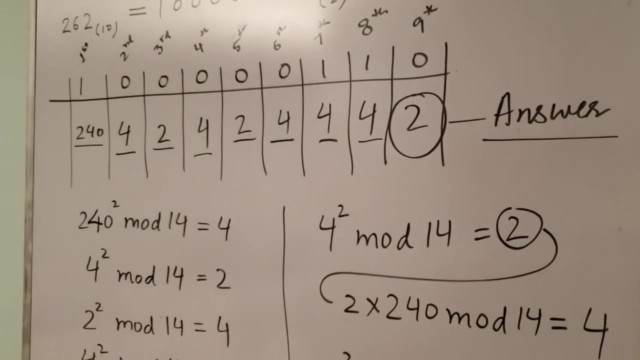 2. Write down 2 in 9th column. So, whatever the value, you will get in 9th column. that is your answer. Subtitles by the Amaraorg community. 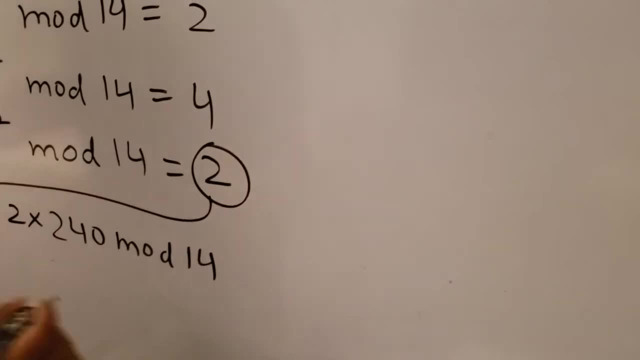 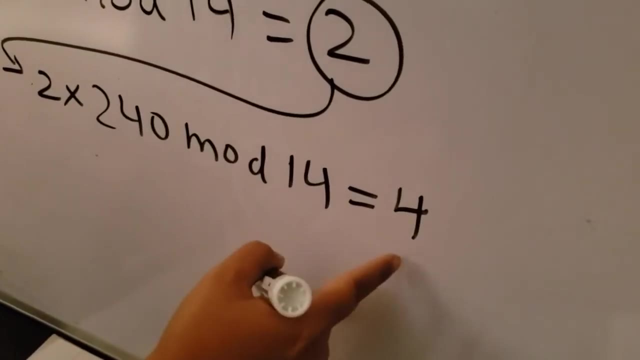 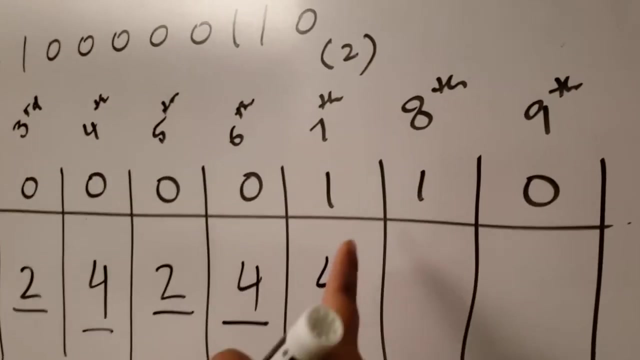 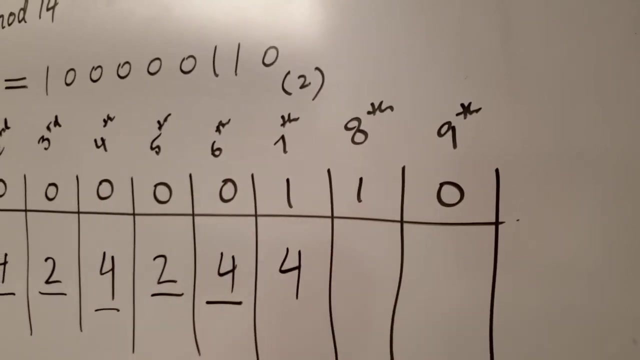 14 owania, you will get the answer four. so you get the value 4 here. write down four in seventh column. now let's look at the binary digit of eighth column, which is again one. now you have to do the two step in this stage, comechtd. 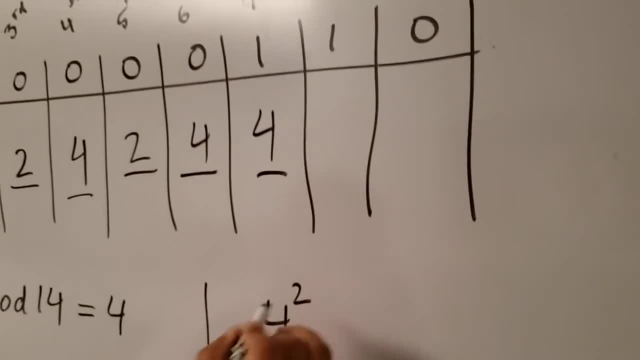 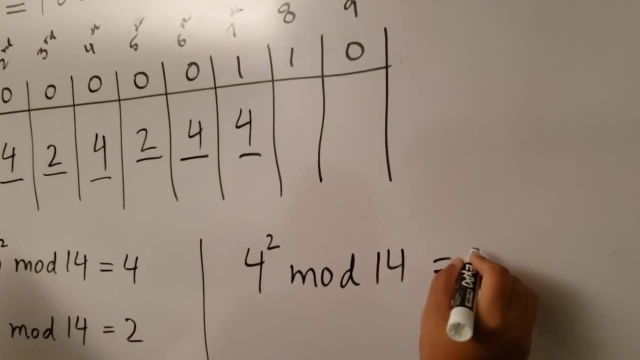 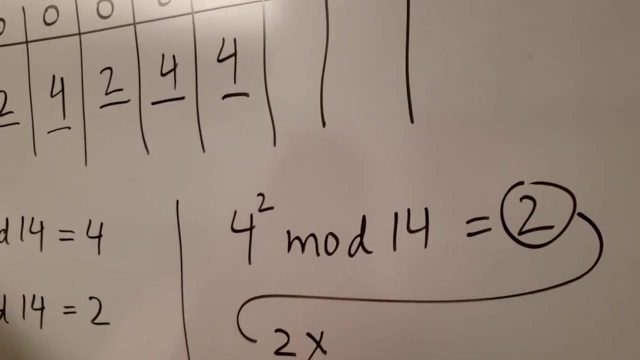 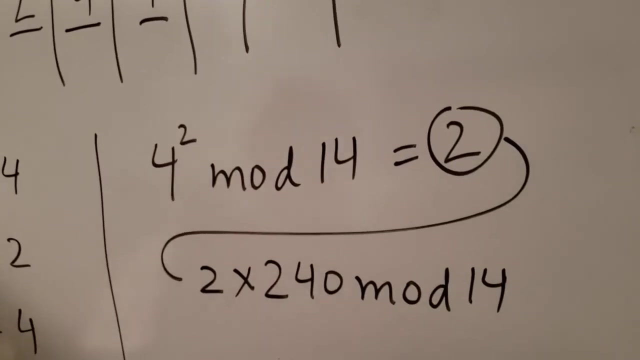 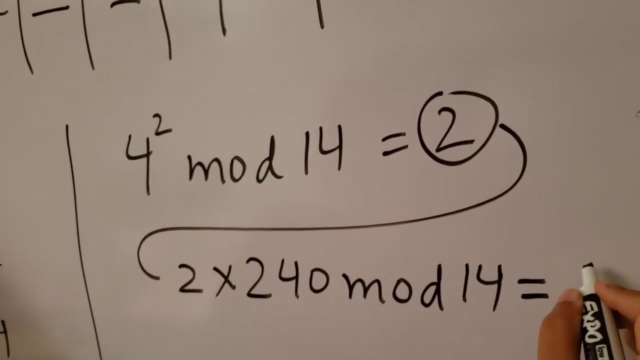 So take 4 square, mod 14,, which is equal to 2.. The second step is: take this 2, multiply it by the base 240,, mod 14. And you will get 4.. Write down 4 here. 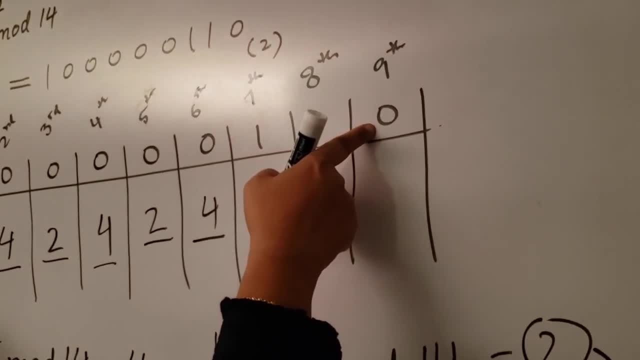 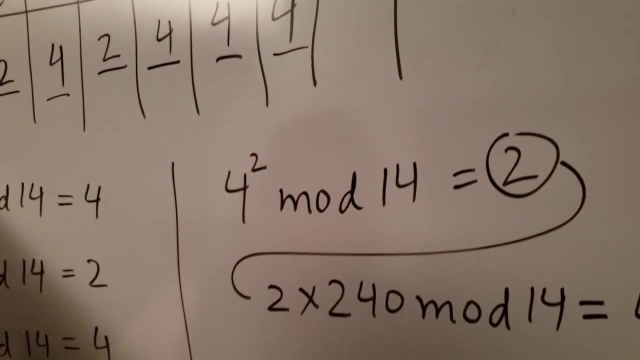 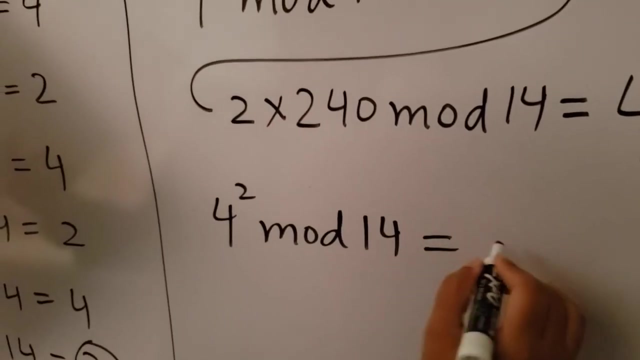 Now let's look at the binary digit of 9th column, which is 0.. That means now you have to do one step. Take the value 4, square it, Mod 14.. You will get 2.. Write down 2 in 9th column. 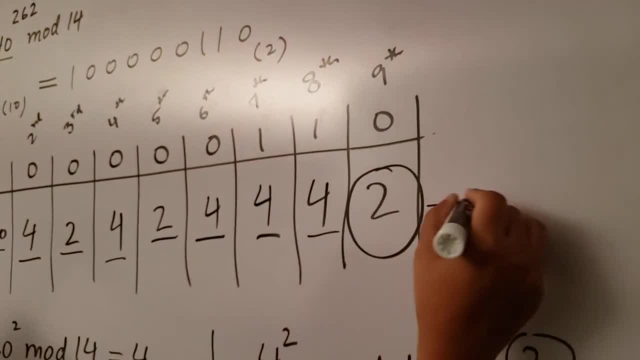 So, whatever the value you will get in 9th column, that is your answer. 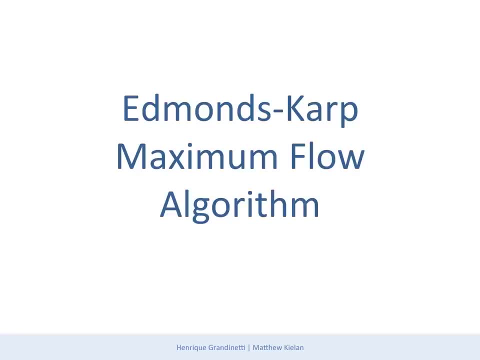 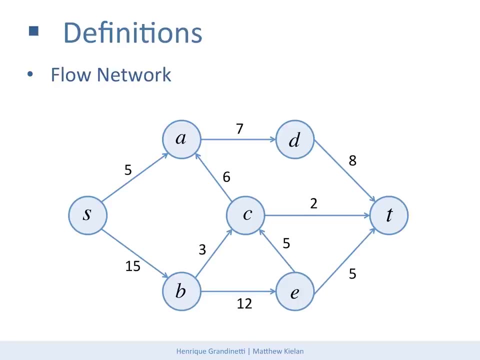 This is an e-lesson prepared by Enrique and Matthew, and it's about the Edmunds-Karp maximum flow algorithm. What is this algorithm used for? It is used for finding maximum flow in a network represented by a directed graph with weighted edges. This corresponds to some real-life problems, such as: 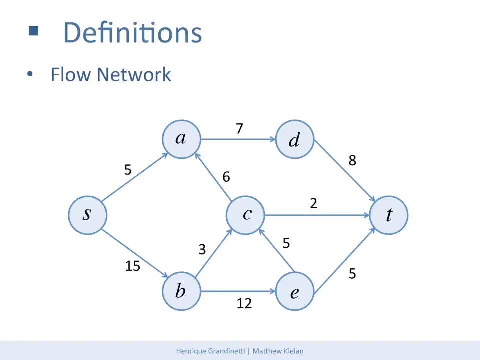 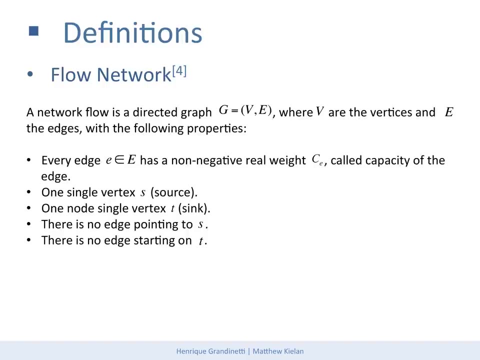 finding the maximum possible bandwidth between two computers and a mesh network where packets can travel along any route independent of each other. Before we discuss the problem in more detail, we need to grasp the definitions of all the concepts involved. So a network flow is a directed graph.